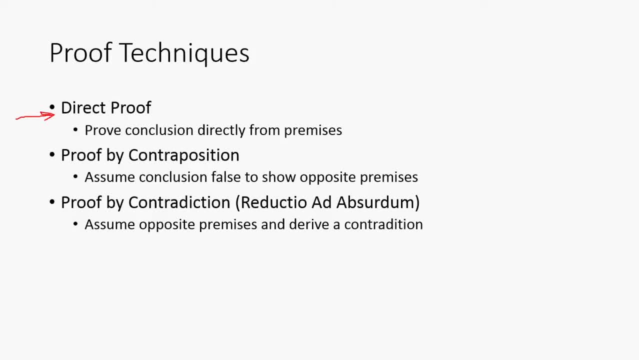 So that was the direct proof, And then next we have our proof by contraposition. So this is where we assume the conclusion to be false, not Q, And then we want to show, not P, Because this is logically equivalent to P implies Q. 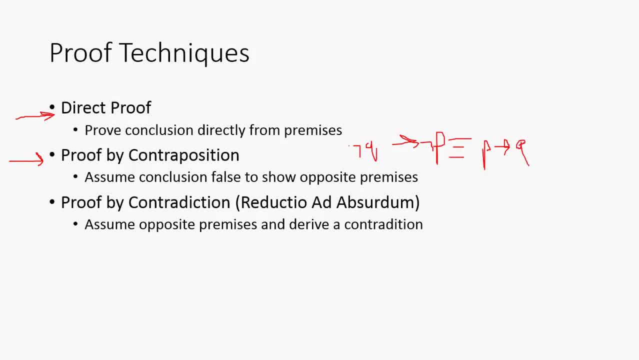 Like so, Okay, So, and then finally, we have our proof by contradiction, also known as reductio ad absurdum. So this is where we assume premises that are the opposite and then we derive a contradiction. So that's proof by contradiction, and we'll show you that in a second. 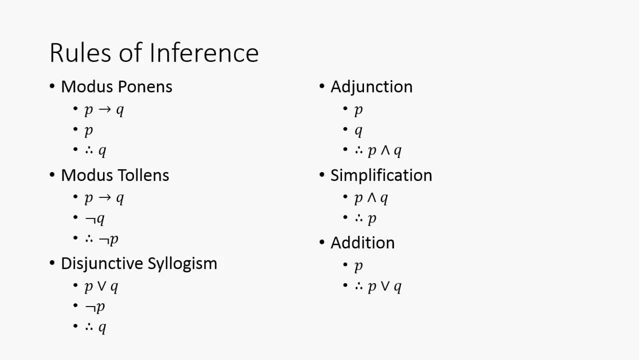 So here are some of the rules of inference. So one of the biggest ones that we'll use is modus ponens, That would be, P implies Q, P therefore Q. Another big one is modus tollens. So P implies Q, not Q, therefore not P. 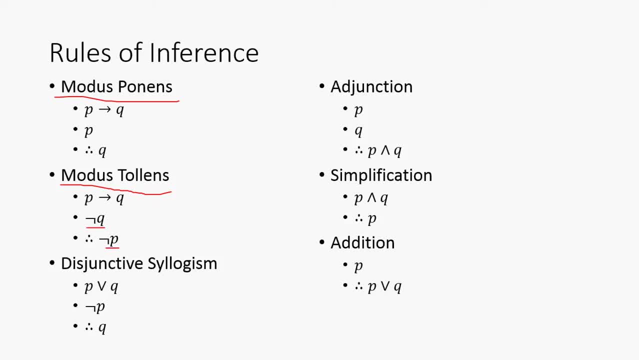 Disjunctive syllogism: P or Q, not P. P therefore Q. That's also a good one Adjunction. This is kind of illustrating the point that each line of a proof is kind of being anded together. 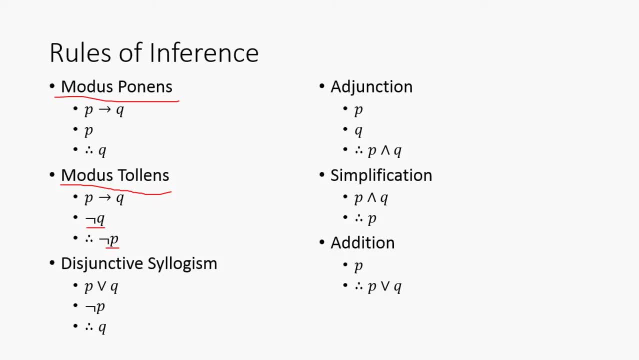 So P, Q, therefore P and Q is adjunction, And then, conversely, simplification is going to be P and Q, therefore P. Since P is true and Q is true- at least they're assumed to be true- then just P is going to be true. 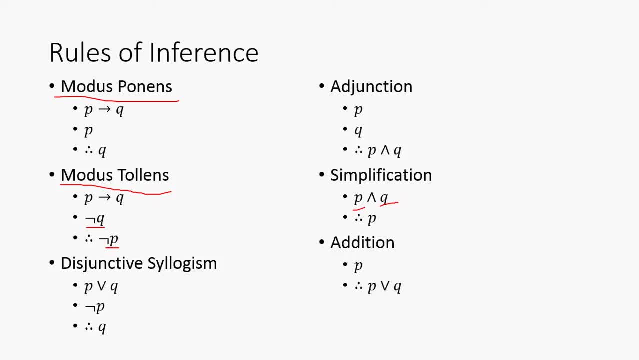 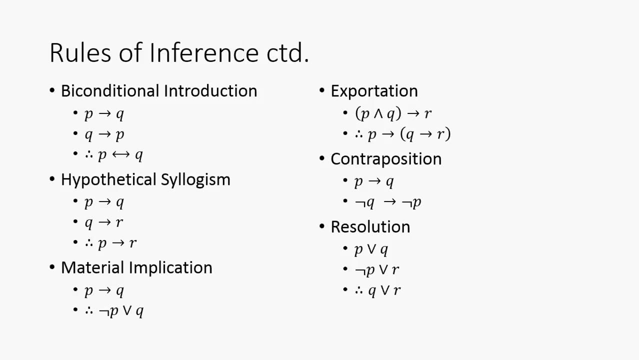 If P and Q is true, And then addition, Because P is assumed to be true, adding stuff onto it like or Q, isn't really going to affect it because P is already true. So continuing on, there's a biconditional introduction. 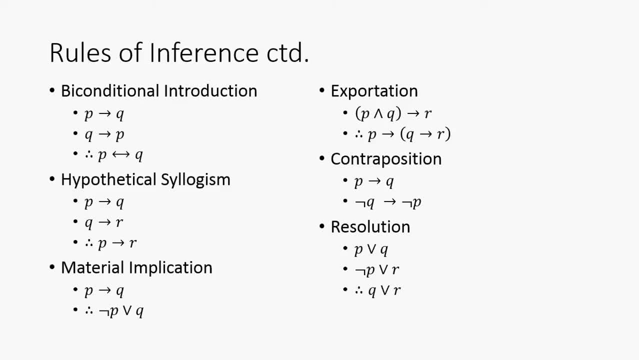 So P implies Q and Q implies P Creates P if, and only if, Q. That makes the arrow go both ways. Another big one is the hypothetical solution: Syllogism. So P implies Q, Q implies R, so the Qs kind of cancel out. 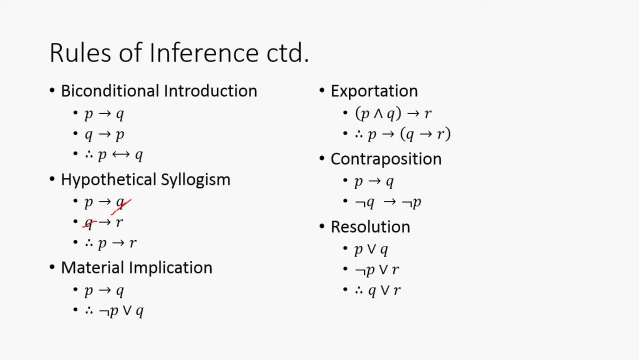 It just goes straight to: P implies R. You can think of it that way. There's also the material implication: P implies Q. This is logically equivalent here to P, if not P or Q, And I discussed that earlier. We have exportation, which is P, and Q implies R. 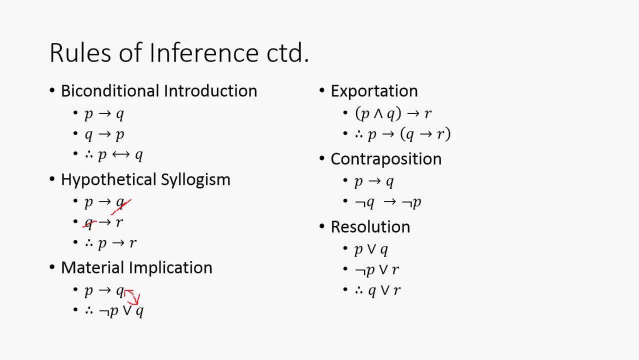 This is equivalent to: P implies quantity, Q implies R- Contraposition. we discussed that earlier And then resolution. So P or Q and not P or R. We can eliminate the P because it's opposite is present in the next premise. 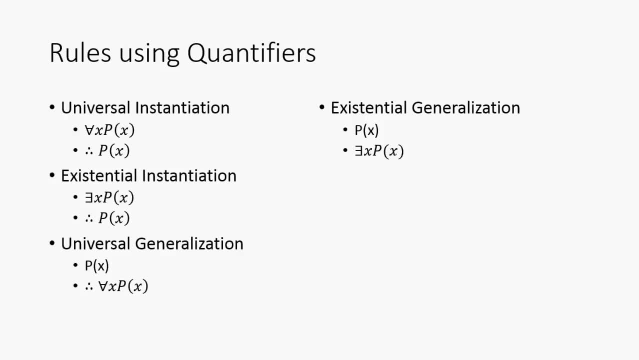 So Q or R. So then there's also some rules using quantifiers. There's universal instantiation, which is where we say for all X, some proposition or some predicate, P of X is true. So we say therefore P of X. 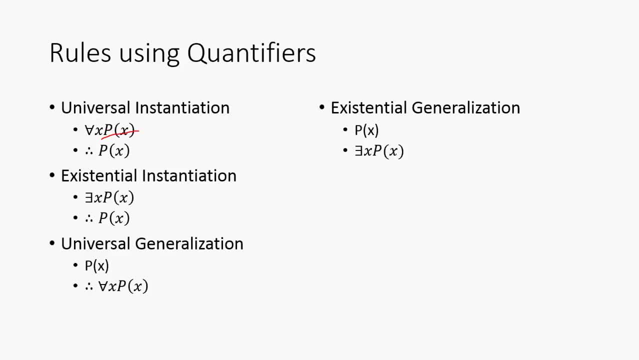 There's also existential instantiation. There exists an X such that P of X, therefore P of X, Universal generalization. This P of X, therefore for all, X, P of X. This is sort of like in the opposite direction of instantiation. 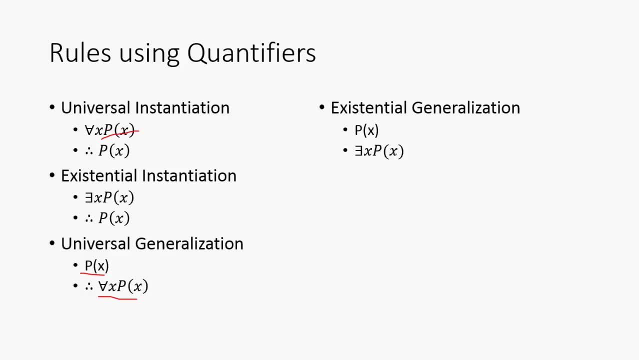 There's also existential generalization, P of X, right. Therefore there exists an X, P of X. So this one totally cool, And then universal instantiation totally cool. These first two are great. You can use them pretty much liberally as you want. 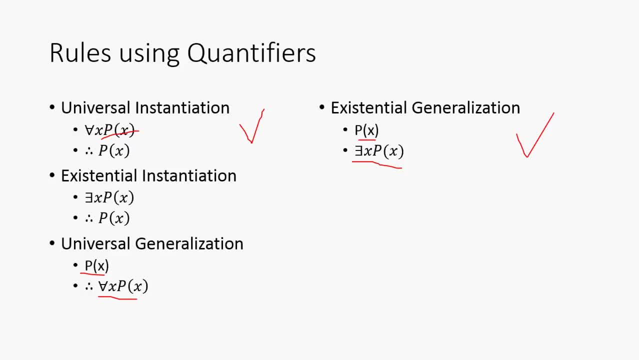 You start getting to like a gray area. You try to say something. therefore all P of X has to be chosen arbitrarily, So in order for this to work, And even then this is kind of an iffy. This is kind of a way of doing things. 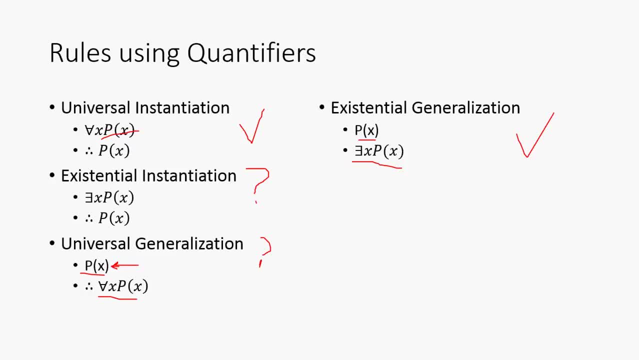 Same with this guy right here Saying that there exists something, therefore there exists an X, such that this happens. Therefore this is going to be true. That's also kind of iffy, But because what if it's not the right X? 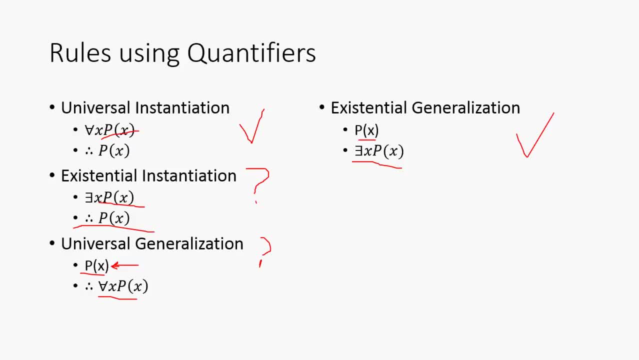 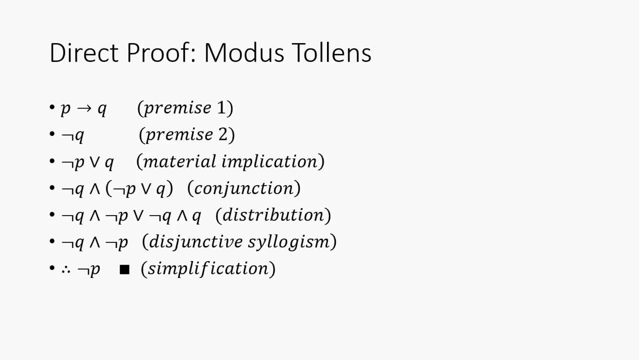 But we'll just go with it. So you just have to be careful using these, So careful. So here's an example of a direction, Direct proof using modus tollens. Or sorry, we're going to be proving modus tollens here. 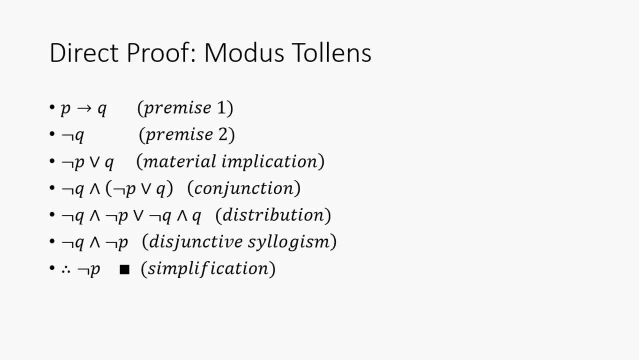 So we have P implies Q as our first premise, Right, And then we'll have not Q as our next premise. So we use our material implication to transform P implies Q into this guy, right here And now. we just use our conjunction law to put these on the same line. 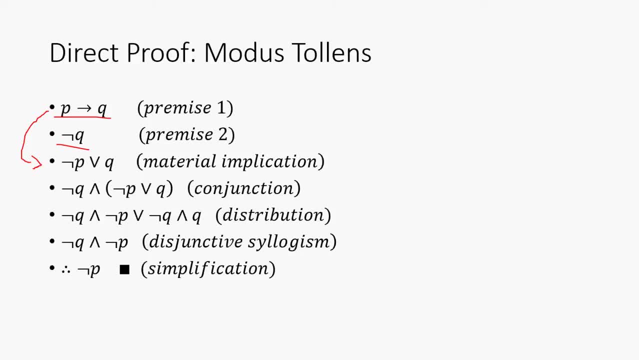 Okay, So we just put that guy right there In combination with this one, Then we just use the distribution law to distribute it out, And then we use a disjunctive syllogism to get rid of this or right here. 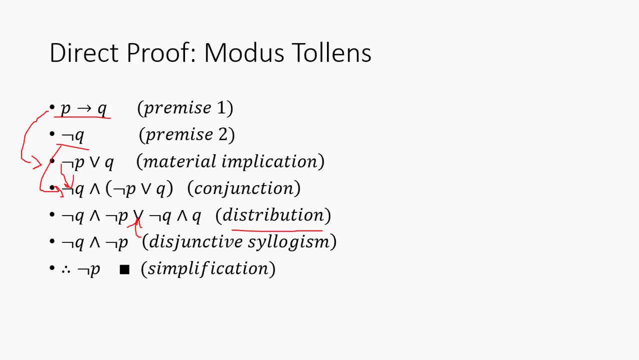 So we have not Q and not P, And then we use our simplification law to eliminate this guy right here, So we get not P, Which is what we wanted to show. So this won't be as symbolic, But it's still going to get the point across. 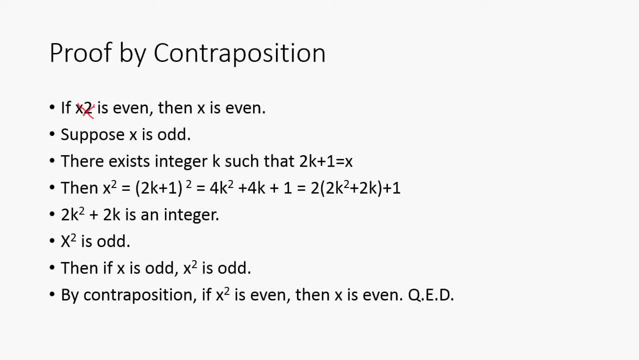 So this right here is actually supposed to be X squared, not X2.. I just couldn't get the superscript working for that one, And even then that's a bad X squared. Just run with it. So we have to prove that if X squared is even, then X is even. 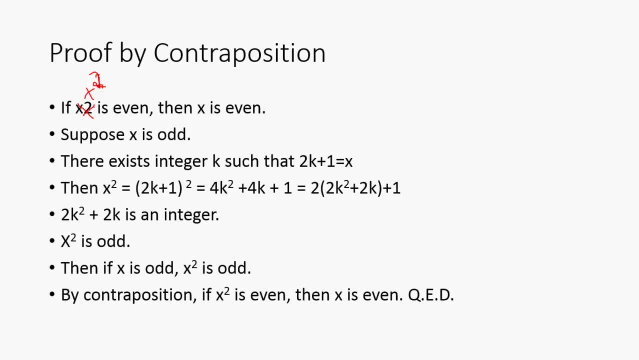 So it's going to be hard to go backwards using this like a square root or something. So instead we're going to suppose that X is odd. So if something is odd, then we use our definition from the last presentation, Such that there exists integer K. 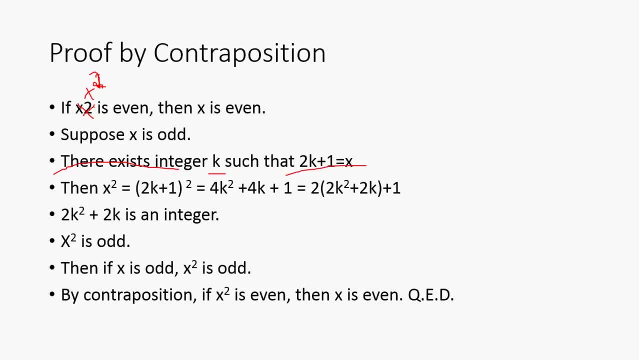 Such that X is going to be 2K plus 1.. Then we just do some algebra. Then X squared is going to be 2K plus 1 squared, Which is 4K squared plus 4K plus 1.. Which is 2 times 2K squared plus 2K plus 1.. 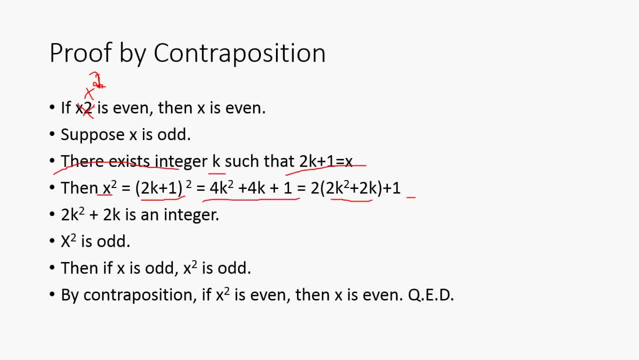 Note that 2K squared plus 2K is an integer, So that's going to be very useful for us. So that means 2 times some integer plus 1 is going to be X squared, Which then means that X squared is odd. 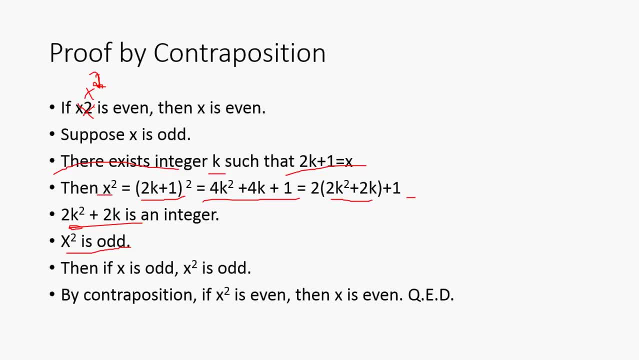 So, using contraposition, this is just a direct implication. So if X is odd, then X squared is odd, Which is what we've just shown. Then by contraposition, if X squared is even, then X is even. 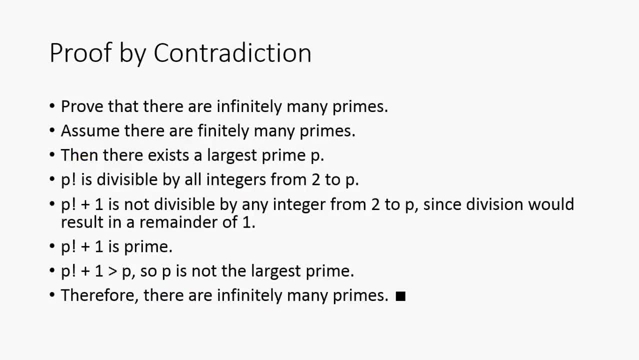 This is what we wanted to show, And then next we have our proof by contradiction. So this is going to be the famous proof done by Euclid, I think, Or Euler, One of those guys. So we're going to prove that there are infinitely many primes. 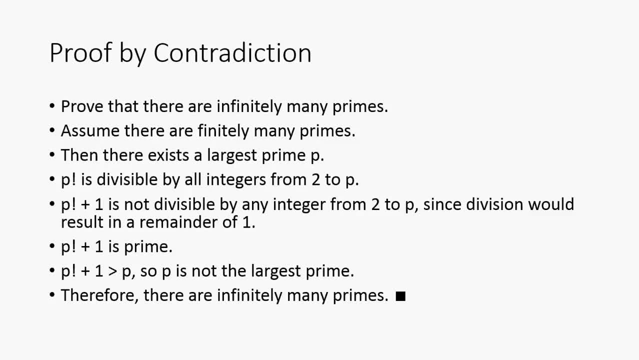 So here we're going to assume the opposite. Assume that there are finitely many primes. So if there's like a finite number of things, we just choose the largest one, because there has to be a largest one, Right. 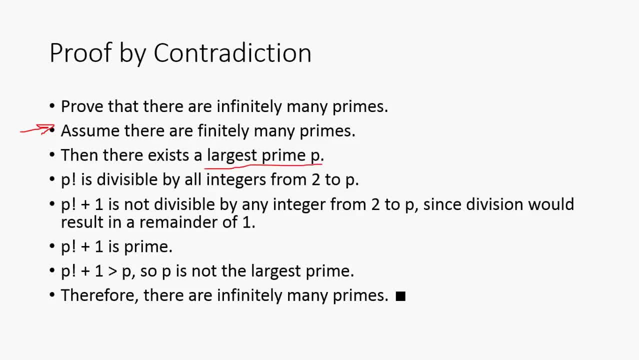 And then we set that equal to P. So P factorial. if you remember what factorial is, it's going to be P times P minus 1, times dot, dot, dot all the way down to 1.. Right, We're just multiplying all the numbers from 1 up to P together. 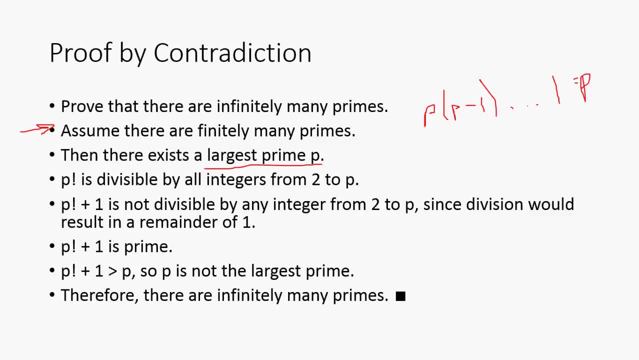 That's going to be equal to P factorial, Right? Okay? So then P factorial is divisible by all integers from 2 to P. Obviously, because that's just how P factorial is defined: It's just all the numbers from 2 to P multiplied together. 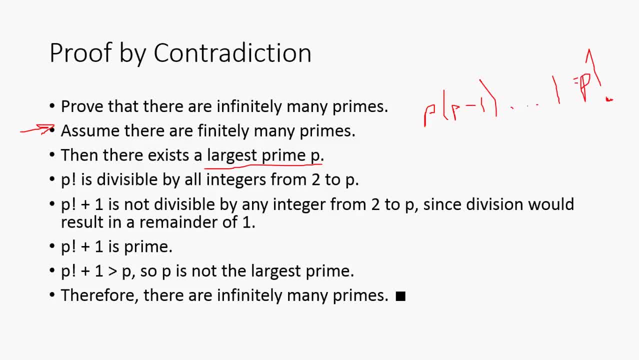 So if we add 1, then every time we divide by each one of those integers, we're going to get our main integer by 1.. So it's going to be a near miss for all of those Right. So then we can't divide. 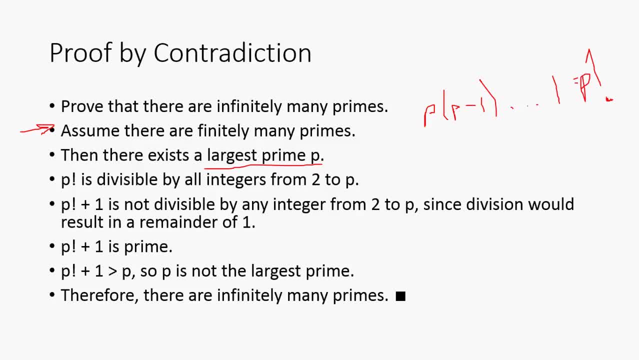 Any of those numbers from 2 to P into P factorial plus 1.. So since none of the primes before it could divide into it, P factorial plus 1 has to be prime. But P factorial plus 1 is clearly bigger than P. 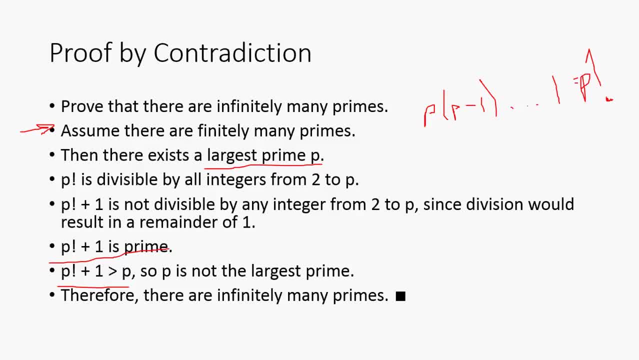 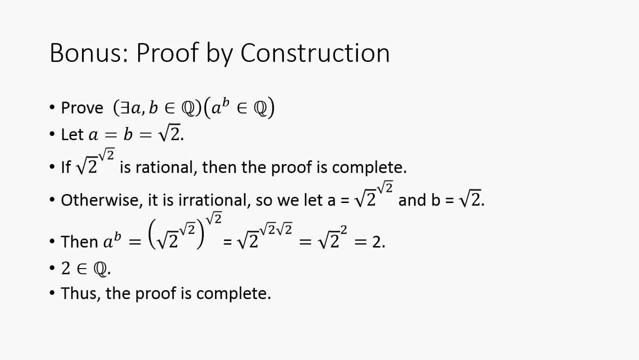 Right. So P can't be the largest prime. Therefore there are infinitely many primes. And here's a bonus proof: by construction, We want to prove that there are numbers that are not rational, such that A to the B is rational. 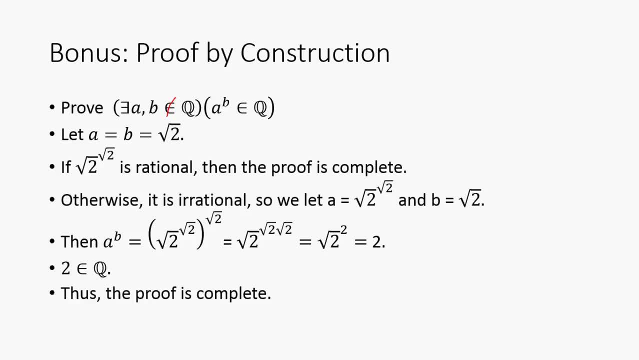 So let A equal B equals the square root of 2.. So square root of 2 clearly is irrational. So if square root of 2 to the square root of 2 is rational, then the proof is complete. Otherwise it is irrational.